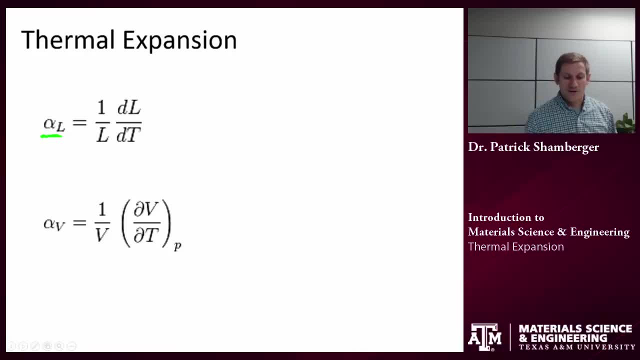 define the coefficient of linear thermal expansion. So that's this term. alpha sub L, as defined as 1 over the length times the change in length per unit temperature. So for every degree Celsius Kelvin Fahrenheit that the material heats up there will be some change in length. So that term 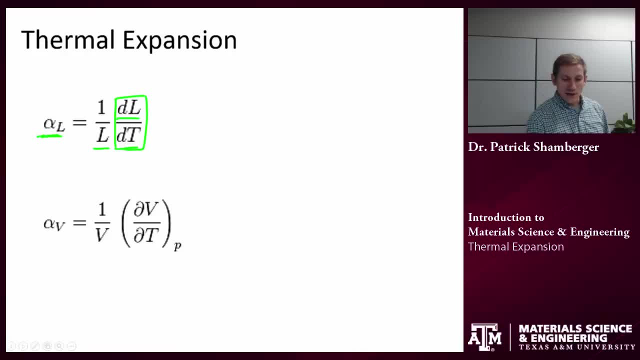 is defined as dL dt. Now let's think about units of the coefficient of linear thermal expansion. very briefly, If I have dL over L, that's going to be the coefficient of linear thermal expansion. Those are both in units of length, so they'll cancel out. So the units of this are given in. 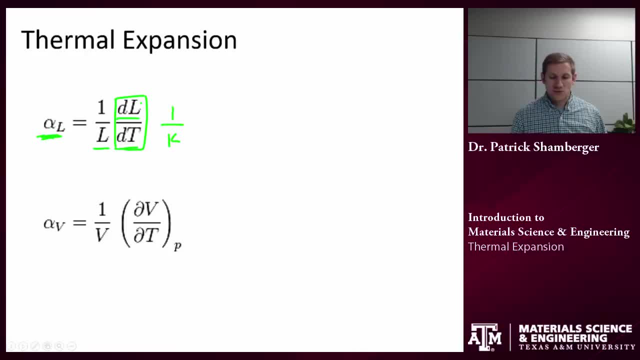 1 over Kelvin, 1 over Celsius, 1 over some sort of temperature unit. Another thing is that we see right off the bat a dL over L term. So let's think back to something else that looks like that. Let's think back to a strain. right, Strain is elongation over total length. If we're talking 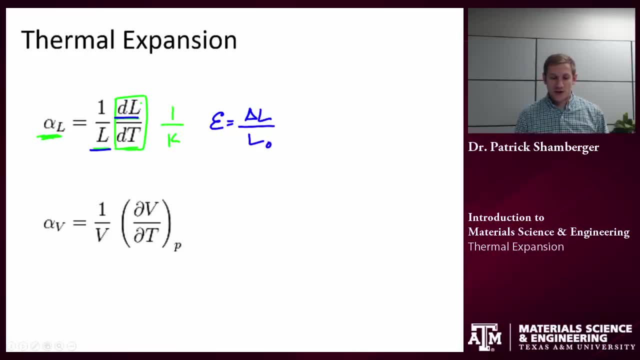 about engineering strain, that's the original length of some material. So I could define, say, a thermal strain in here as well. So another way to rearrange this expression would be to say: alpha dt equals some thermal strain, right, If the linear coefficient of thermal expansion is? 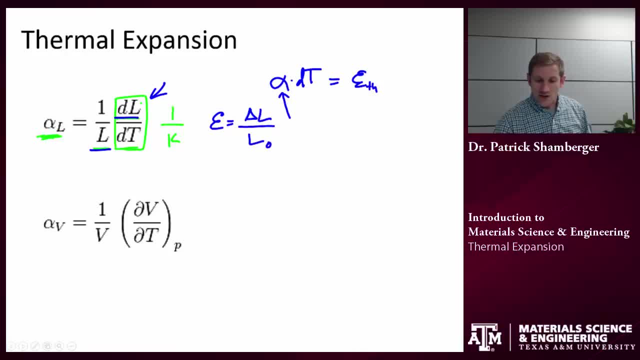 relatively constant over some temperature range. then I could replace dt with a macroscopic change in temperature, temperature difference, right? So alpha delta t Equals thermal strain. Okay, so why is this important? Well, let's think about some part. 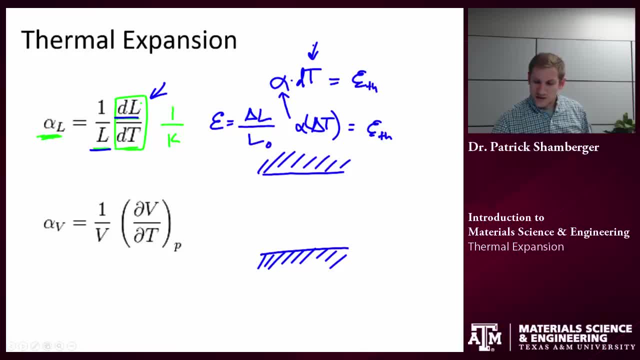 And I'm going to have that part confined. So here's some sort of top barrier and bottom barrier And here's the part. Now, if I heat this part up, it's going to want to expand, And the expansion that it would want to see is given by this expression here, right? So let's think about. 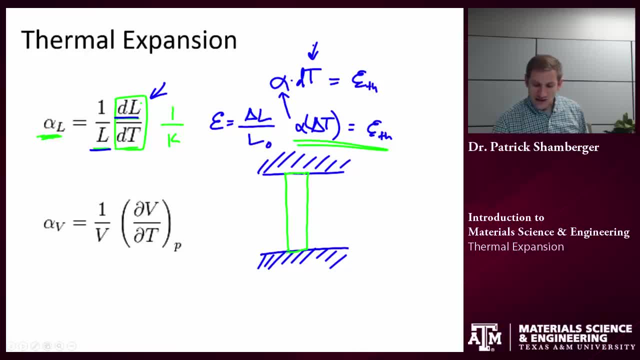 if this bottom barrier wasn't here. If it heats up, it's going to want to expand, And really I'm only thinking about this expansion in the one direction, So the linear coefficient of thermal expansion. However, we know that this barrier is here, So what happens is that 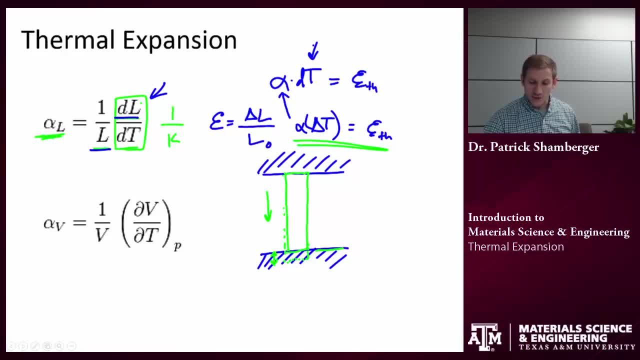 the barrier is supplying a force and ultimately a stress back on this component. I'm pushing back on the component In the opposite direction so that it retains its its original length. And so the way we would figure that out is we would look at a stress strain curve and say 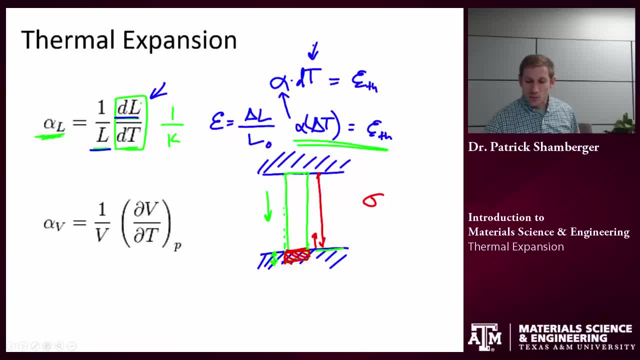 what sort of stress is needed to apply to counteract that thermal strain? right, Because the two strains have to be equal if there's no net change in length. So this is why we care about thermal expansion. So there's also a volumetric expression. 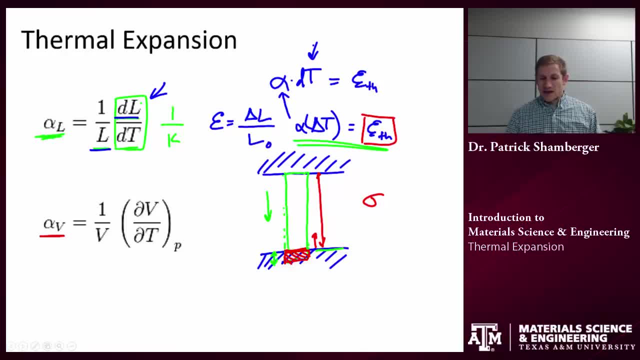 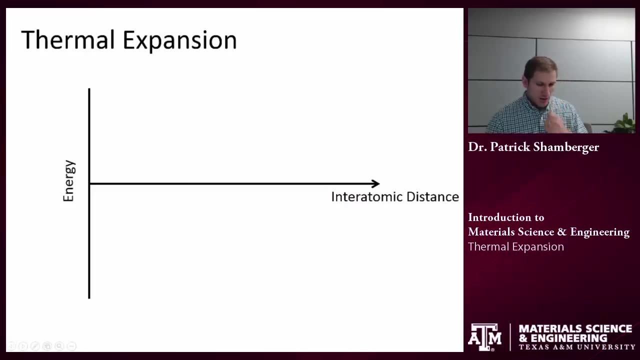 definition because if it's expanding in all directions, there would be an overall volume change. So you can occasionally see a volumetric coefficient of thermal expansion and that's defined very similar. Now, where does thermal expansion come from on the atomic level? You'll remember that we talked about 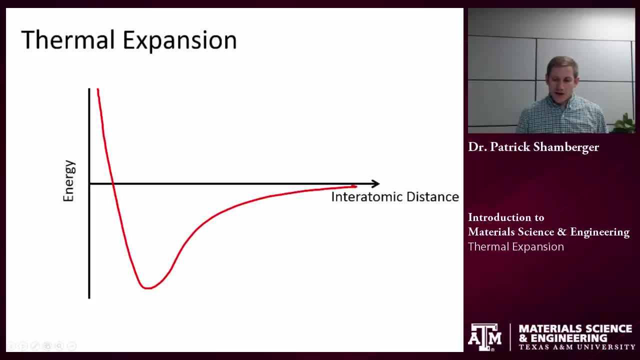 bonding curves before right And this is looking at the bond between two atoms and we're plotting the energy versus the inter-atomic distance, so versus the distance between those two atoms. So we said before that at zero Kelvin the equilibrium distance is going to be given by that energy minimum, right? 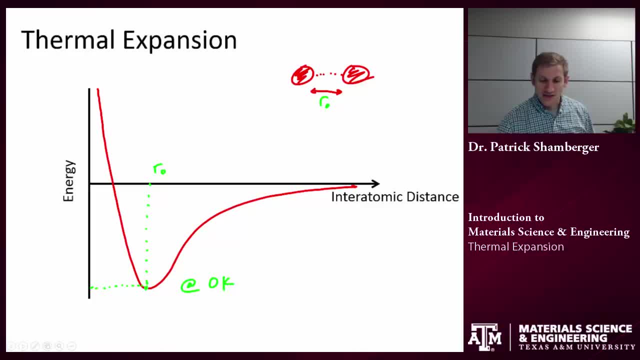 So I would call this R naught. That's the equilibrium distance. So that's if there's no temperature in the system. But what happens as the system starts to heat up? As I heat up the system, I'm giving it more kinetic energy, So now I'm able to access slightly higher energy levels. energy. 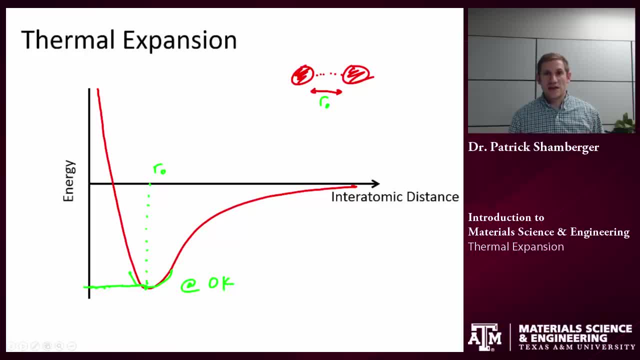 levels between those two atoms. So in other words, if I heat it up, the atoms are able to start vibrating to some extent, so that the total energy can be a little bit higher than it was before. So let's say I give it some thermal energy. 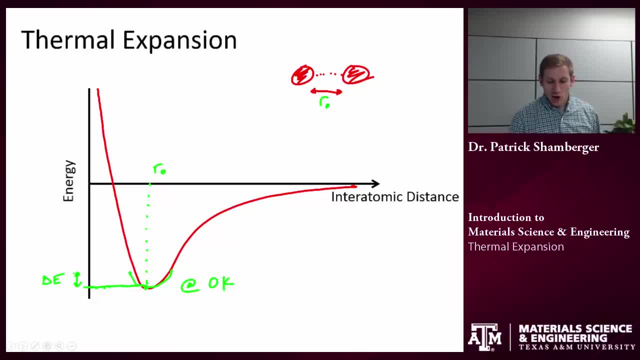 that's equivalent to R naught. So that's the equilibrium distance. So that's the equilibrium distance. So that's the equilibrium distance. So now the atoms are able to vibrate back and forth between these two positions, And so I could consider what is the average position of those two. 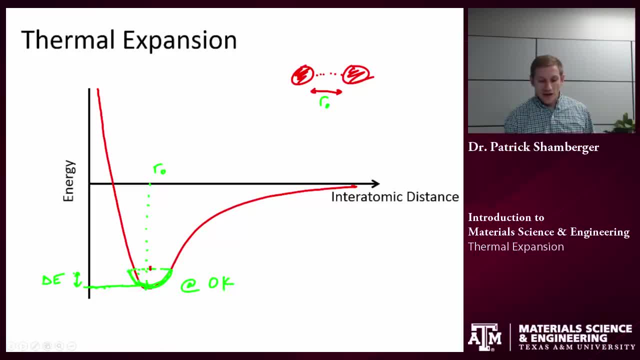 atoms, And if I say that they're equally likely to access any of these states in between, then that average is going to bisect the distance between these two points. Let's heat it up some more, right At this point. now I can actually. 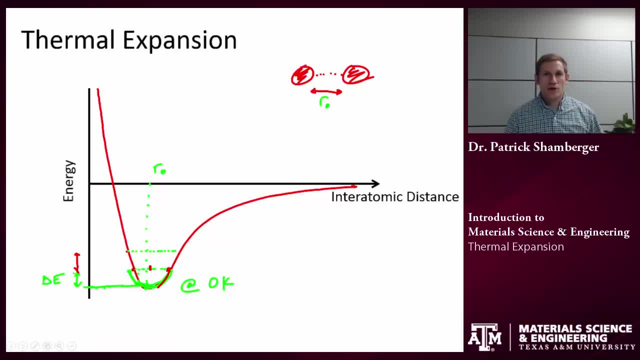 and access an even wider inter-atomic distance. The more thermal energy I'm putting in, the larger I'm able to get these vibrations to swing. So at this point the average inter-atomic distance would be somewhere over here, And if we keep doing this process again and again, 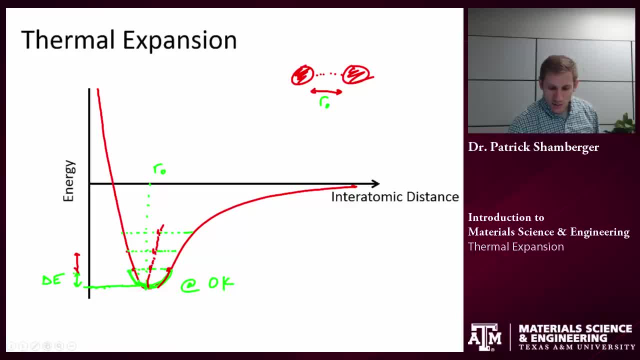 what you'll start to see is that the equilibrium thermal distance is getting longer and longer, And this is exactly what causes real materials to heat up. right As I heat it up, this curve is always asymmetric. If I had a perfectly symmetric bonding curve, 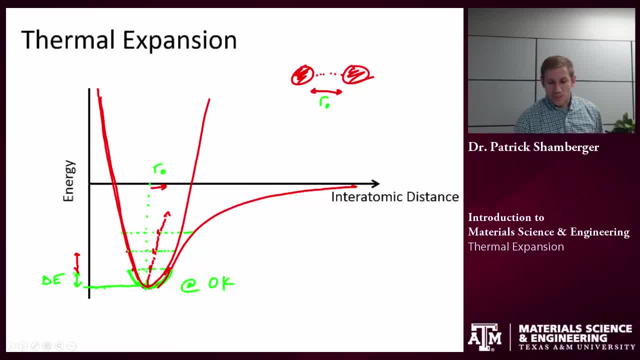 then I wouldn't expect materials to heat up, But, by virtue of the fact that there's a finite distance, that they can come together and they could go infinitely far apart, it is an asymmetric curve. Okay, so let's think about another thing. 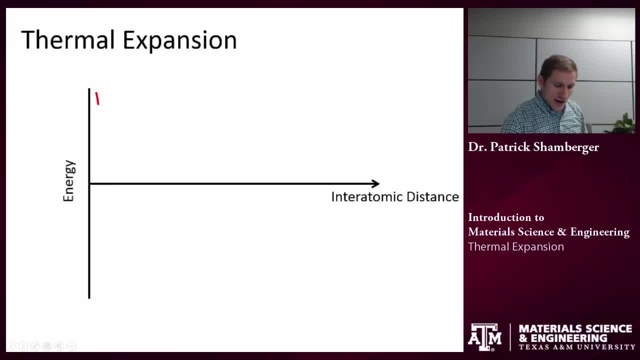 Let's think about, let's compare, two materials. one has a relatively strong bond, and so strong bonds are given by relatively large energy wells, right. So the other bond will be relatively weak. So one example would be something like a diamond or a tungsten, something that has a very 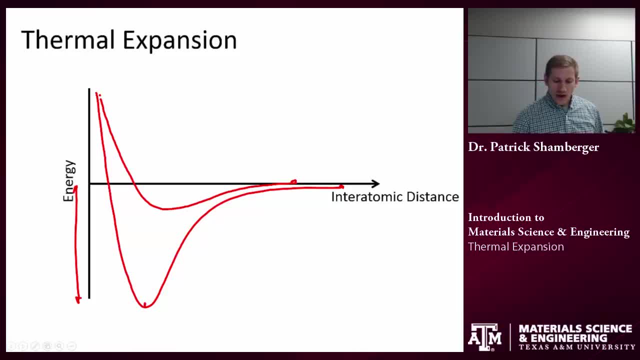 it's a very refractory material, really high melting point. Something with a weak bond would maybe be the Van der Waals bonding in between polymer chains. Now, if we do this same procedure, if we heat the material up in both cases, we'll start to see something pretty interesting. 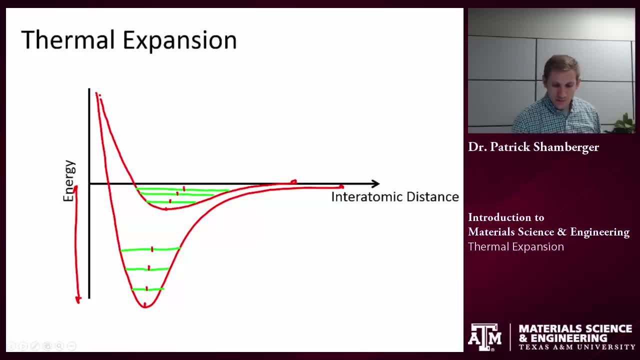 And that is that for a smaller amount of heating we tend to get a larger change in equilibrium distance in the weaker bond. Then we do, Then we do, then we do in the stronger bond, in the stronger bond. So again, this is the weaker bond.